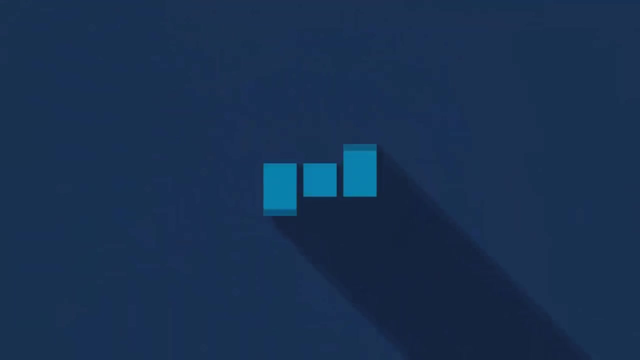 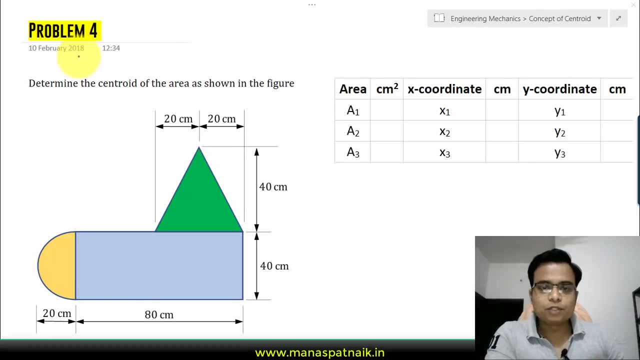 Hey guys, what's up? this is your friend and tutor Manas, and it's gonna be yet another session in this lecture series on engineering mechanics. Well, today we're gonna be continuing with our discussion on centroid calculation and, in that regard, we have taken this problem and this. 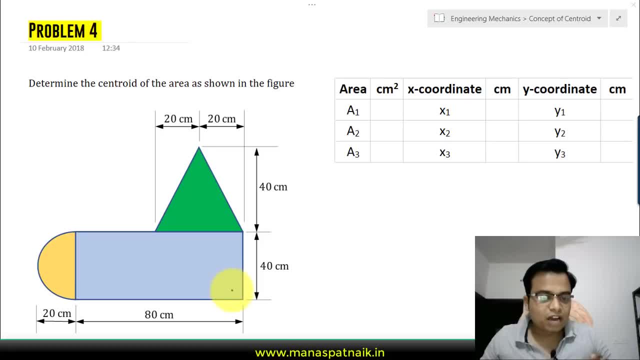 basically is a combination of different geometric figures. So we have a rectangle- let's say this is one- marked by one. let's say this triangle over here has been marked by two, and we also have a semicircle. Now we have to find the combined, combined centroid of all of these figures. 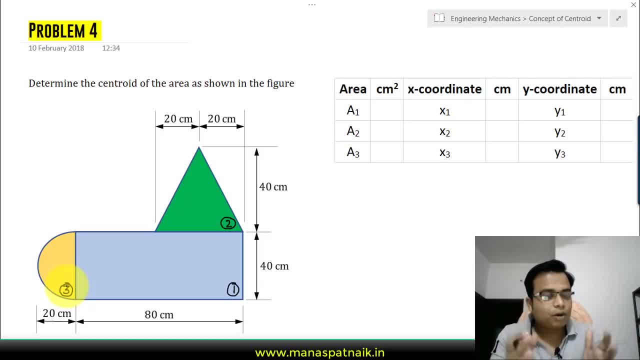 right taken as a whole. Well, how can that be found out? Well, here is the approach. So initially we will be calculating their areas individually. So let's start with rectangle. so its area will be 80 multiplied by 40.. 80 multiplied by 40 is pretty simple. that's 30 to 100. 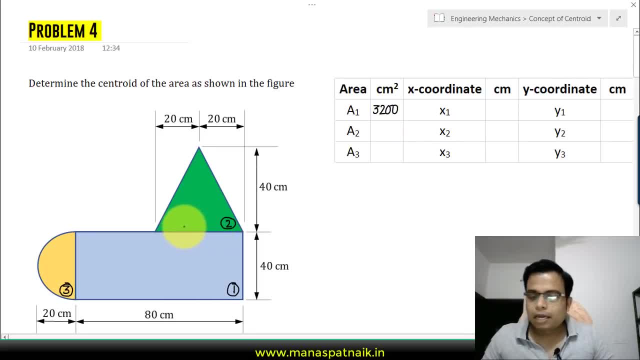 Secondly, you have this triangle over here and you know very well the triangles area is given by half of base into height, So a2. if I were to calculate the value of area of triangle, it will be half of base. This base from here to here, it's how much? 20 plus 20, that's 40 multiplied by this height from. 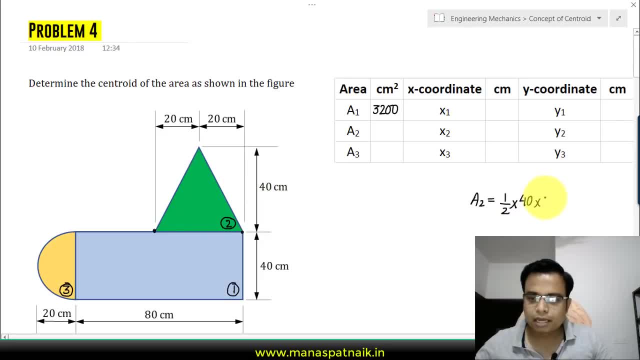 this point. to this point, that's 40. okay, and this is also pretty simple. this is gonna work out as well. And then, finally, we have to calculate the area of the semicircle. you can see very well that this semicircle is symmetric about this line that I've drawn just now. okay, about this horizontal. 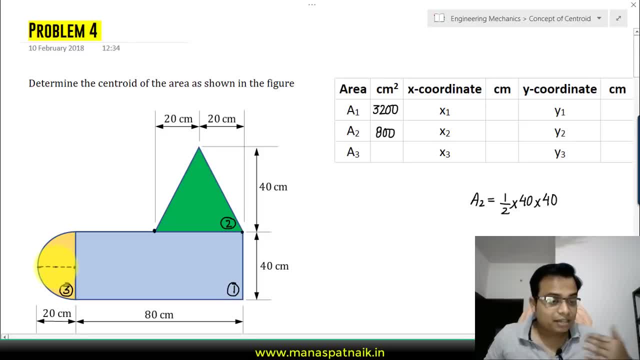 line. Now that has no connection with the area. I don't know why I said that, but you can clearly see that the radius of this semicircle is 20 centimeters. okay, and if I were to calculate its area, its area is going to be equal to pi r square. pi into 20 square. but hey, that's the area of a. 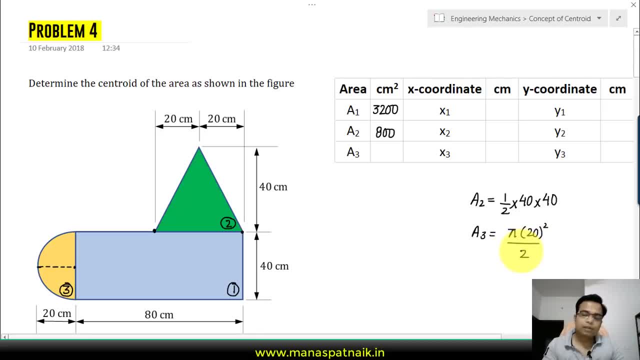 semicircle, and when you divide it by 2, you will get the area of its semicircle. Well, put that up into a calculator and then you're going to get the value of the area of semicircle as 628.31- 628.31. 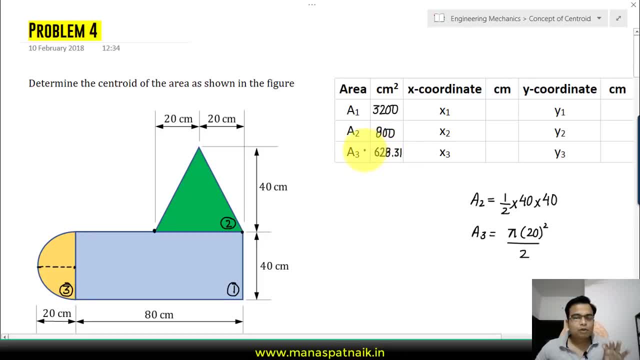 done. Now what? now we'll do an individual analysis for all the three geometrical shapes, okay, and then we'll try to calculate their x and y coordinates, form of x 1, y 1, x 2, y 2, n, x, 3, y 3. but for carrying out all these things, what I really 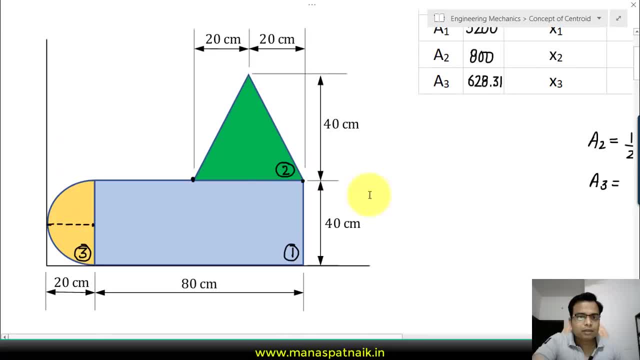 need is a coordinate axis. so the coordinate axis has been, has been made right and- let's say this over here- represents the y axis and- let's say this over here, represents the x axis. now, now, the center of this geometrical figure, this blue one right, this is 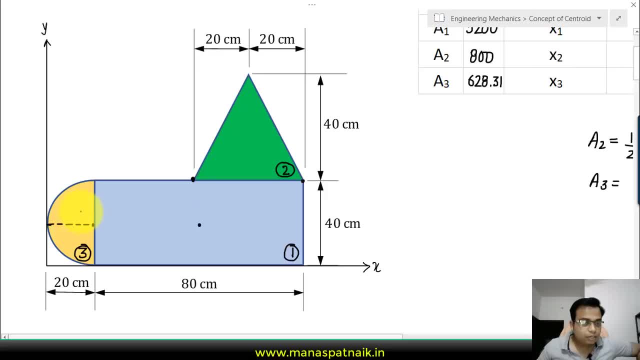 in fact, a rectangle will be somewhere here. okay, and if I were to tell you this will be x 1, x 1, right, and this over here will be y 1. this pen appears to be a very thin. let me have a thick pen. so how can x 1 be calculated? now, guys, from this point to this point, this is pretty simple. 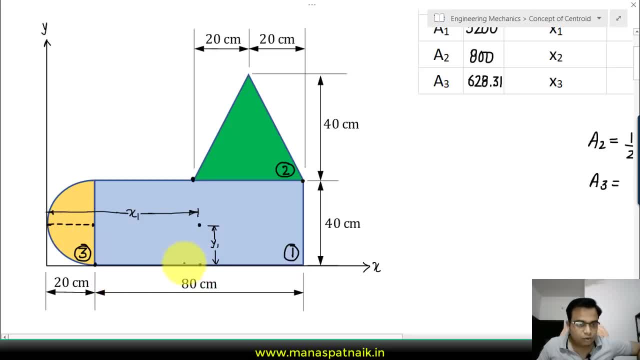 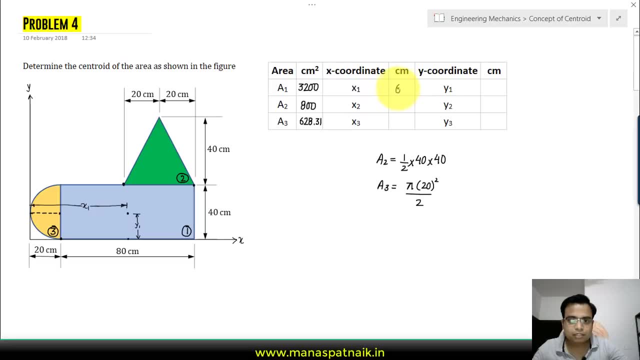 half of 80, that's 40. and when you add 20 to this 40, you have the value of x 1. okay, so x 1 is nothing but 20 plus 40, and that's 60. let me just write 60 over here. that's it. let's again focus on y 1. what? 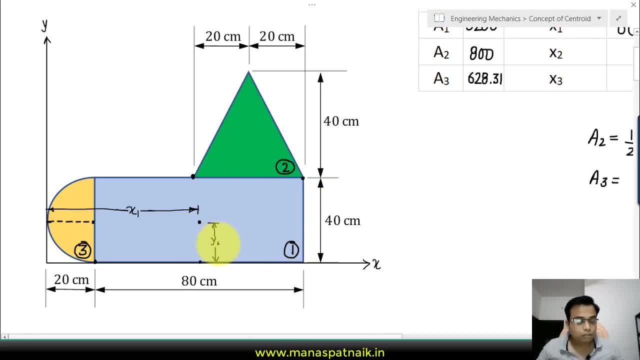 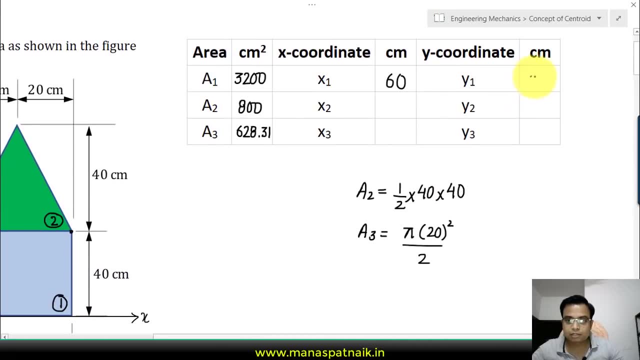 about y 1. so the height is 40. so half of 40 is going to be the value of y 1 and y 1 is going to be 20. okay, that's pretty easy. so y 1 can essentially be written as 20. so that's 60 and that's 20. now 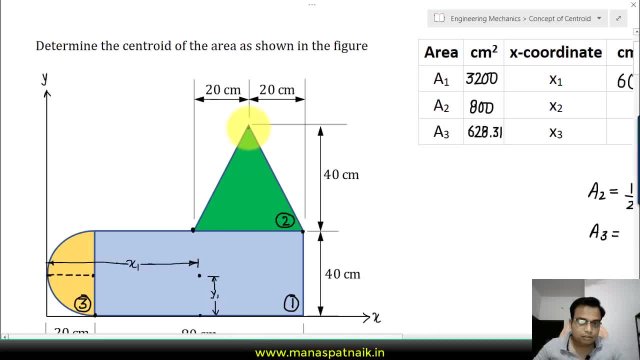 let's focus on this triangle. okay, guys, now remember this: whenever you are dealing with triangle centroid, always try to draw a median from any corner. okay, like this, centroid will be at a height from the base. this height, this height, will be h by 3.. so how much is h for this? it's 40, okay, and 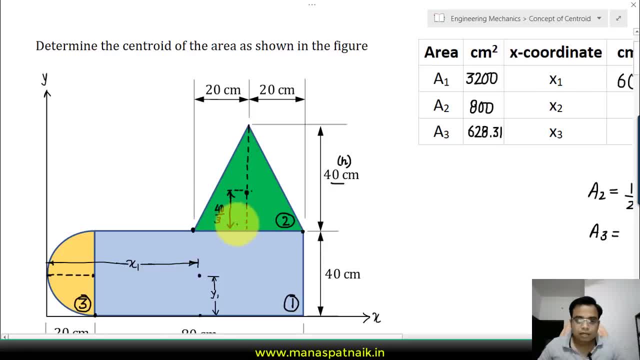 this is going to be 40 by three. now what I'm supposed to find is the value of y 2. okay, so y 2 is precisely this distance. sorry, I cannot, like I'm not able to make this straight line. so y 2 is equal to how much from here to? 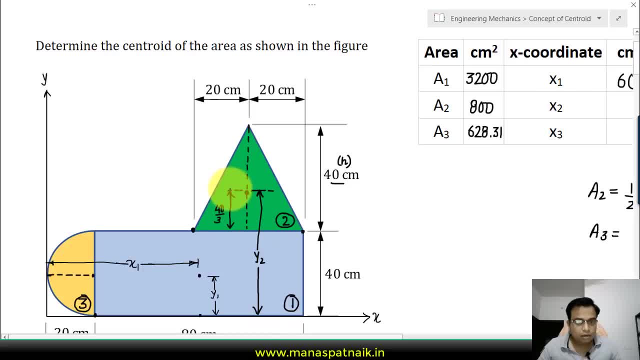 here it's 40, 40 plus 45 in, that's y 2. so when you do 40 plus 45- 3, are you gonna get this value 50, 3.3, 3. let me write here also: y 2 plus 45- 3. so here's the value of y 3. here's the value of y 2. 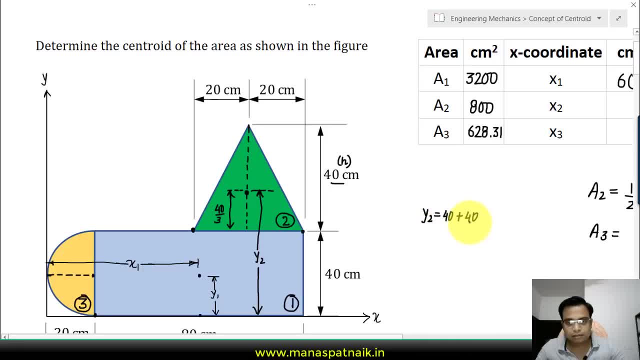 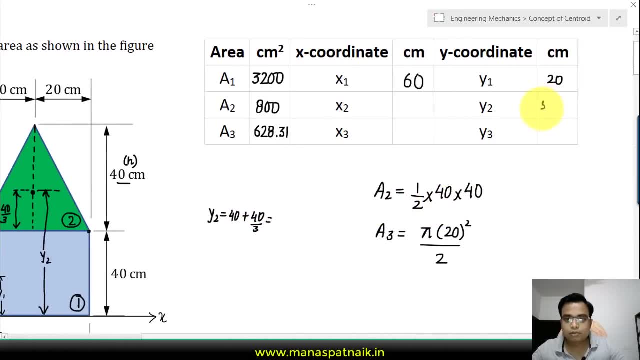 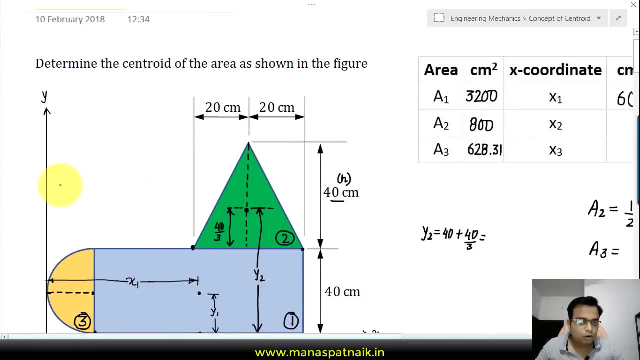 2 is equal to 40 plus 40 by 3. okay, so you put this up into a calculator and you're gonna get 53 point 3, 3, y 2, 53 point 3, 3. now we are interested in calculating the value of X. now, that's X 2. distance of the centroid from the y. 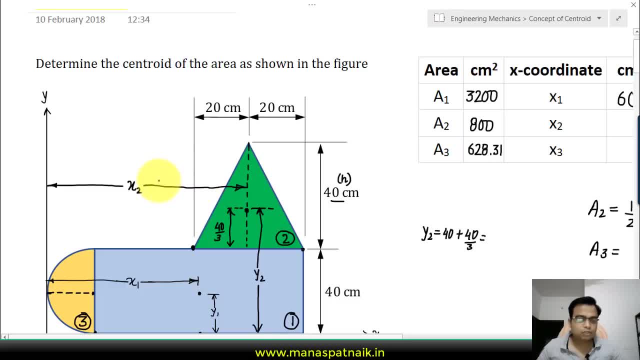 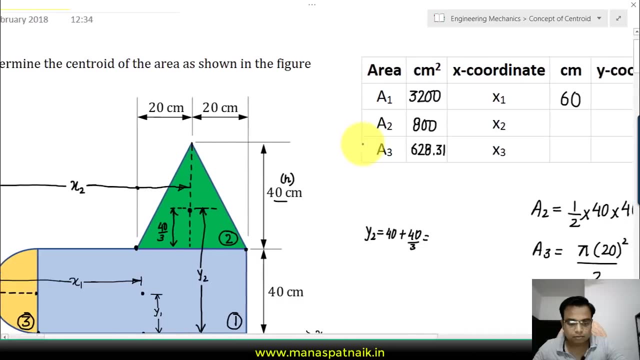 axis, that's X 2. now this is pretty simple. X 2 is pretty easy from this point to this point. the distance is how much? that's 20 plus this 40, 20 plus 40 is 60, 60 plus again 20 is 80. so X 2 is going to work out as 80, pretty simple. 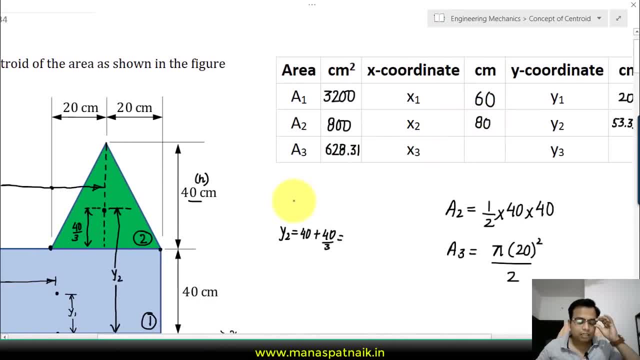 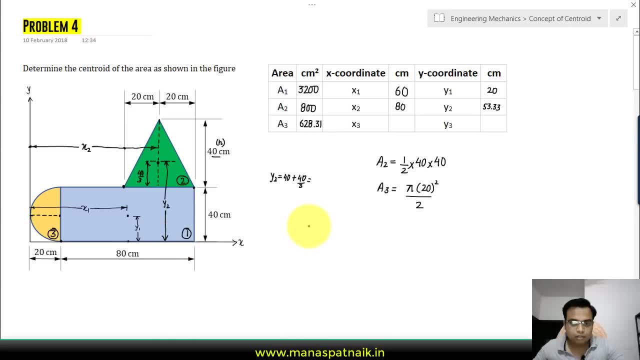 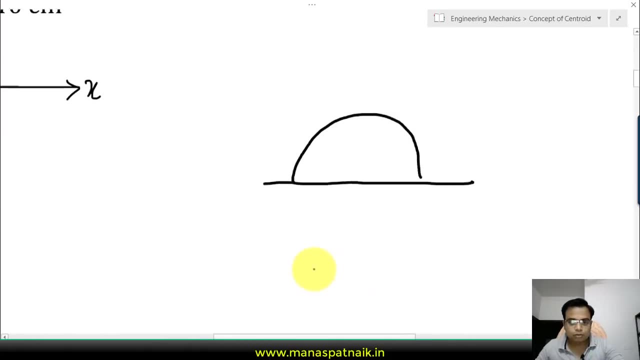 that's 80. and then finally, let's, let's work out for this semicircle. now let me tell you something. I don't know if you, if you're aware of this or not, if you have a semicircle of this sort, let's say: this is the base, right? let me zoom on to this now. the 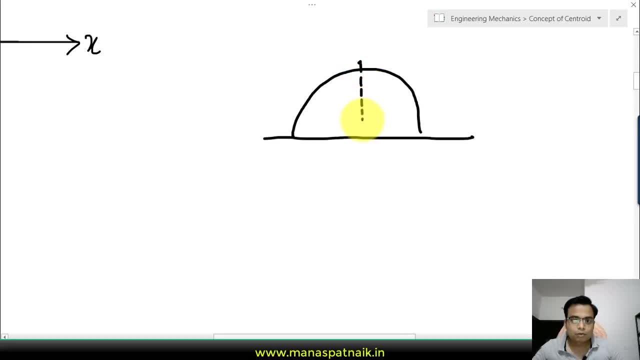 semicircle, first of all, is symmetrical about this vertical axis. okay, over here we have our, this is also our. so the centroid will be at at a height of 4 R upon 3 pi from the base. this is 4 R upon 3 pi from the base. always, even if even. 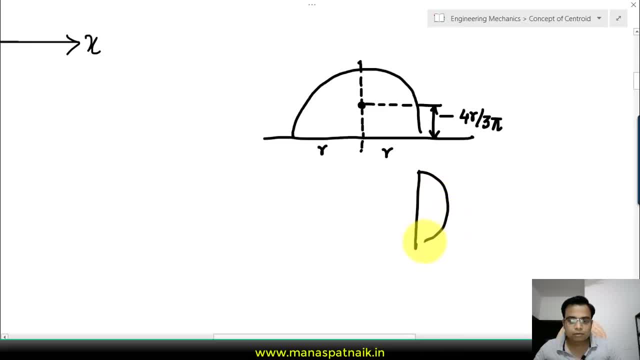 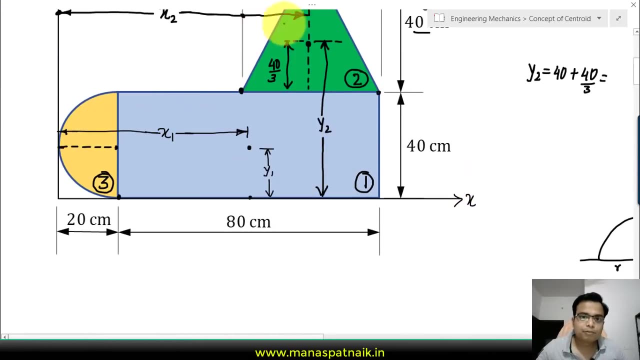 if the semicircle is something of this sort, you okay in that case. also this: this distance always from the base is gonna be equal to 4 R over 3 pi. always remember this. now let's try to implement the same stuff over here. would be better, if I can. 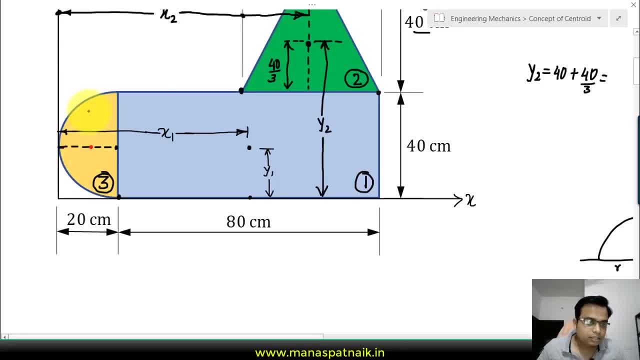 have a different color. it can use a red color. the centroid is essentially going to be somewhere here. now this is gonna be 4 R over 3 pi. what is R? well, the value of r is 20, but what do we need? we need this, and that's what you call x3, and x3 is equal to. 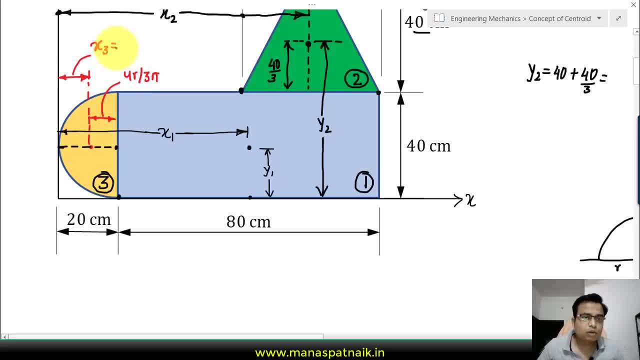 what x3 is equal to how much? that's 20 minus 4r over 3 pi, 20 minus 4r over 3 pi. so you just have to put the value of r, which is going to be equal to 20, put that up into a calculator and the final. 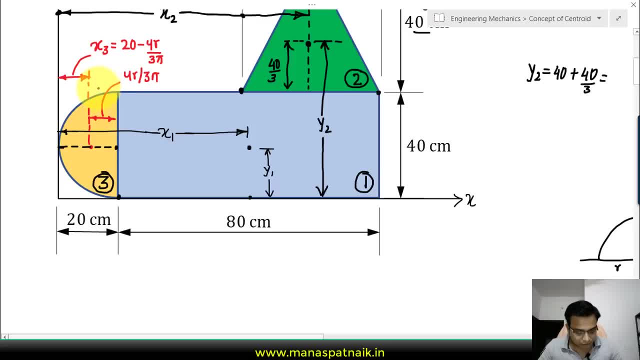 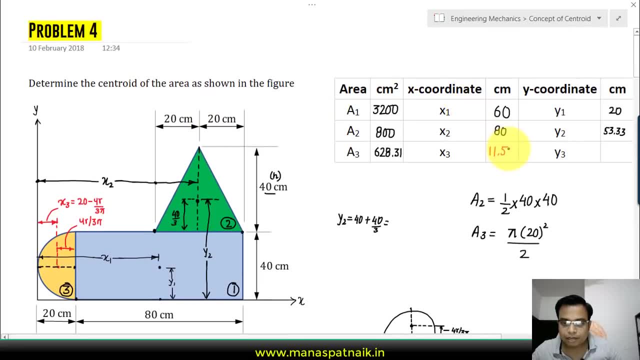 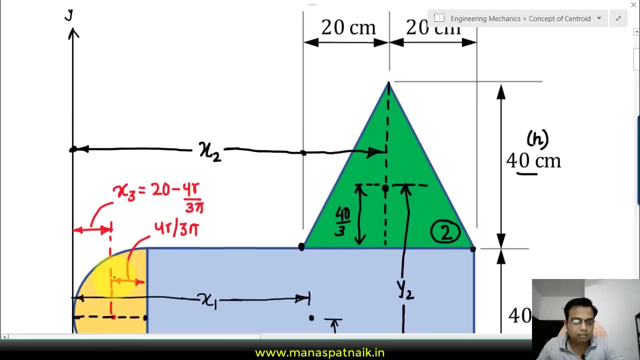 value of x3 that you're going to be getting is 11.52. let me write that: 11.52, 11.52. finally, what's left is the value of y3. well, y3 is pretty simple. okay, it's. it's something like this: this is the. 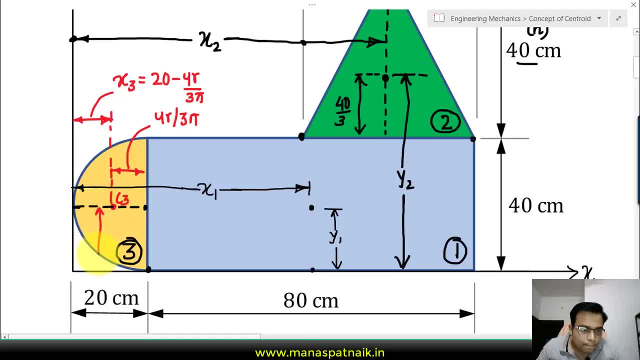 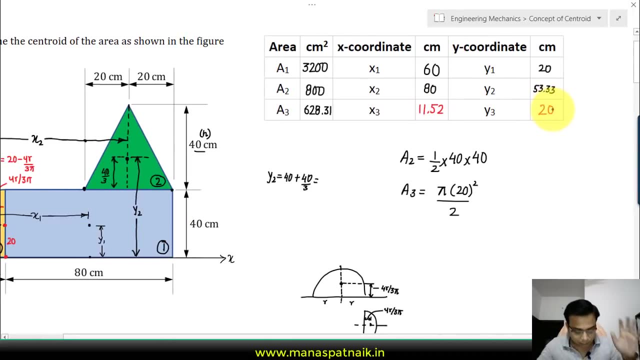 centroid, let's say c3, and this over here is y3. okay, so y3 is pretty simple. how much is this from here to here? that's um 20 only. okay, that's 20.. so the value of y3 is: let me see, that's 20.. now let me go ahead and check. 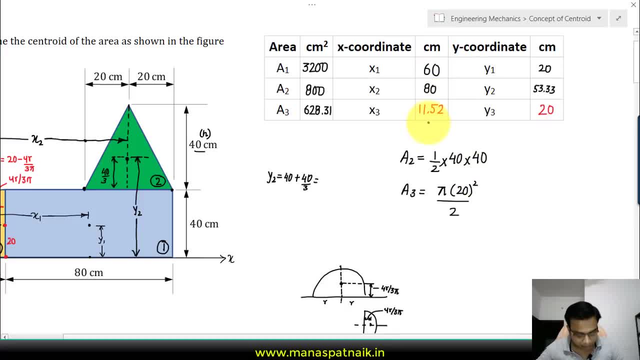 all of this: 20, 53.33 and 20, and this is 60, 80, 11.52. yeah, areas of 3200, 800, 628.31. okay, let me, let me have the eraser. let me, this is it's gonna be doing my job, okay. 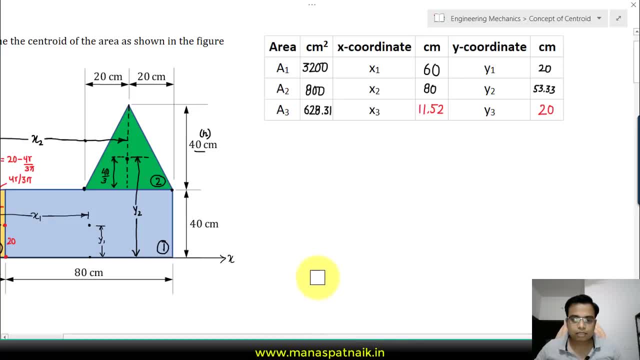 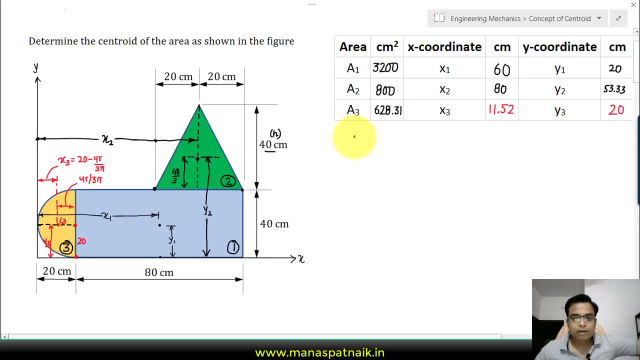 one final step and then we are almost done. all right, now what we are doing is we are finding the centroid of the composite figure, so we are adding all the three geometrical shapes: 1 plus 2 plus 3.. okay, now, what? what? essentially, the formula. 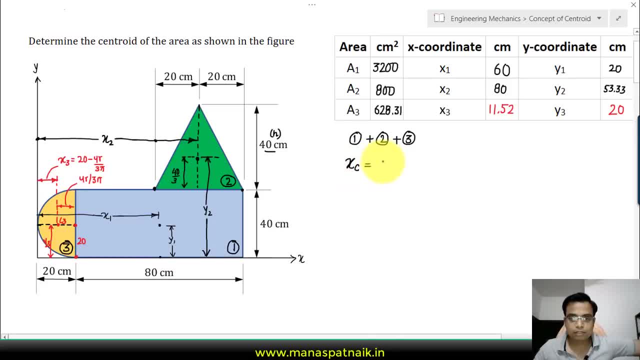 of xc will be the centroid or the x coordinate of the centroid is going to be equal to a1, x1 plus a2, x2, a3, x3 over summation of all the areas. or you can just write simply a1 plus a2 plus a3 in the same.